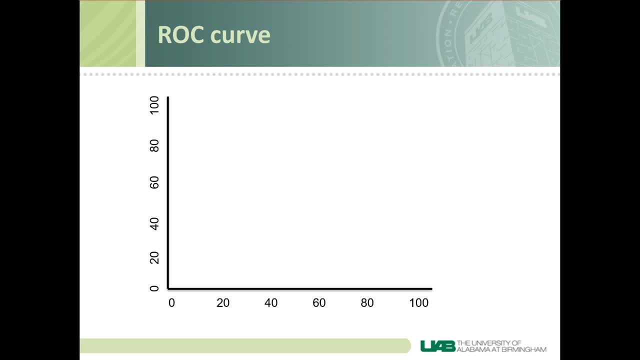 test for the same disorders. I'll show you in a minute. So how do we construct an ROC curve? Well, on one axis we plot the sensitivity of a diagnostic test at a given cutoff points versus one minus specificity. So we plot true positive rate versus a false positive rate. 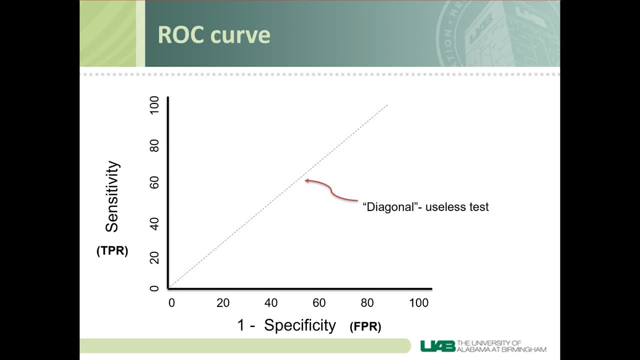 There's a diagonal line that cuts across the middle. that indicates where a useless test would fall, and I'll talk a little bit more about that in just a second. A perfect test is going to along the left-hand side and perfectly horizontally across the top. It has 100%. 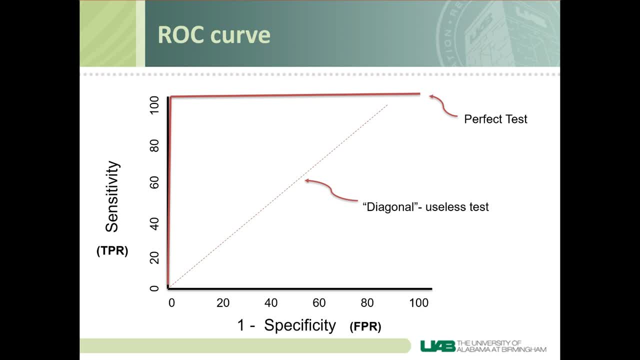 sensitivity and 100% specificity pretty much at every cutoff point. It's rare that you see a perfect test. So how we construct an ROC curve is: we take all the individual cutoff points of a given test and we recalculate sensitivity and specificity for each of these cutoff points. 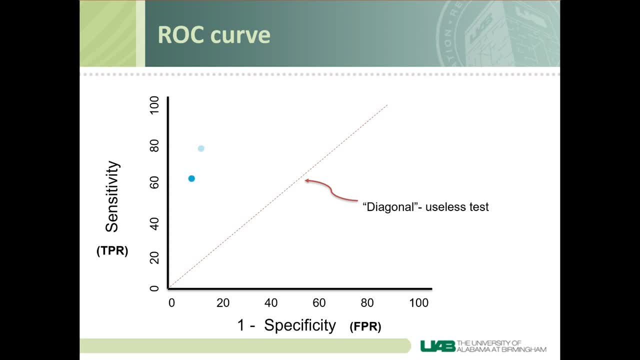 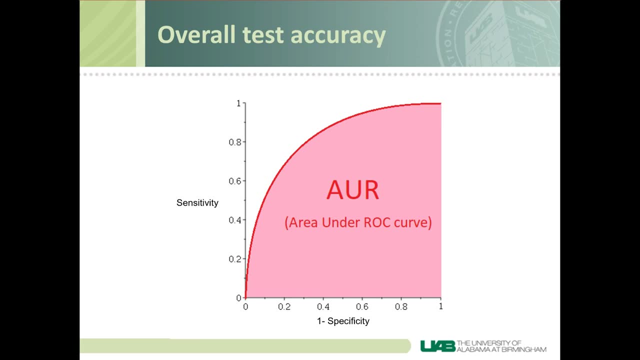 and we plot them on this curve. So we'll plot all the individual points and draw a line through them, as we see here, and that's our ROC curve. Now, I mentioned a minute ago that we can calculate or determine the overall diagnostic accuracy of a test, and we call this the area under the ROC curve, And a best test is the whole. 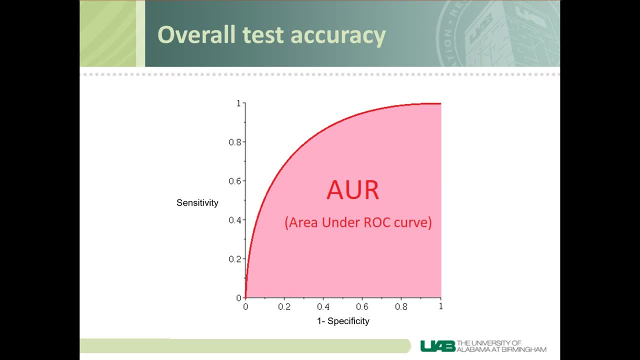 curve is colored in and it gives an overall accuracy of 100%. And as we get less and less and we get close to 50% of an area under the ROC curve and 50% accuracy is useless. It's basically a coin flip and not a useful test. So we want our area under the ROC curve, our diagnostic accuracy. 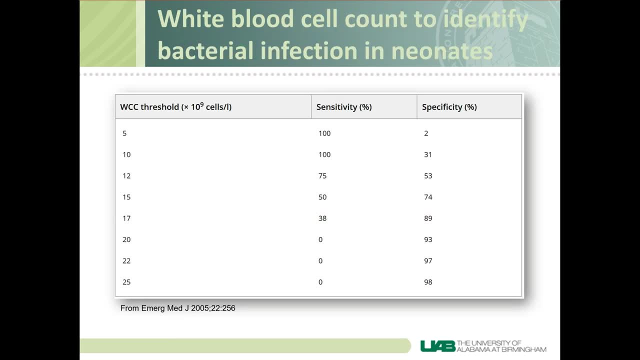 to be as high as possible. So we want our area under the ROC curve to be as high as possible. Let's look at a test or an ROC curve of some real data. So this is data published in the Emergency Medicine Journal in 2005,. 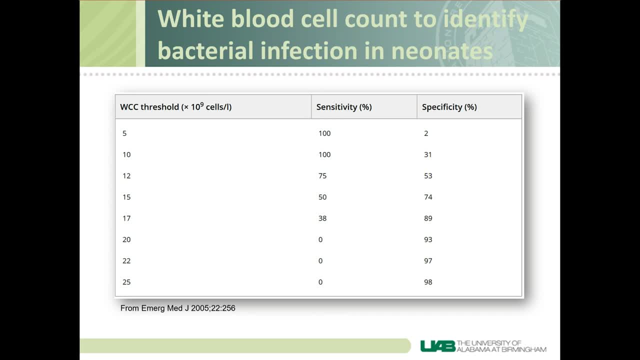 and the authors looked at different various white blood cell count cutoffs for detecting bacterial infection in febrile neonates. Over here you can see the different white blood cell cutoffs and for each of these it has a corresponding sensitivity and specificity. 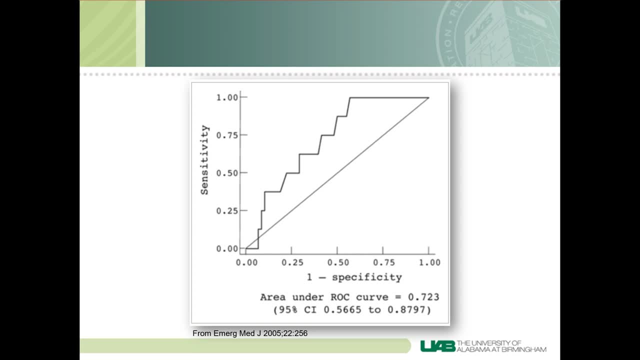 And when you plot these on an ROC curve you get a graph that looks like this. So each of the this curve is all the individual points of those different cutoff points, And so we want to compare noise, as you can see, of tedious control of features, values of white blood cell count, as you saw on the slide.